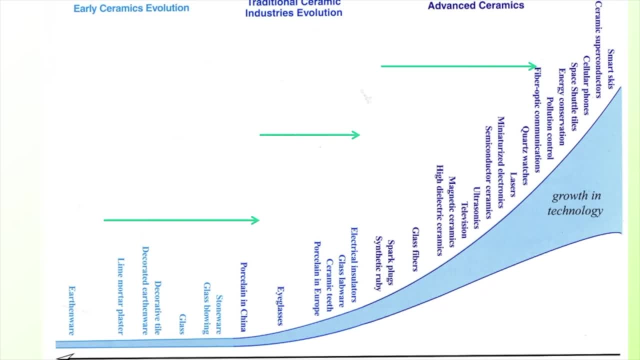 In more detail. ceramics have evolved from very small to large. Ceramics have evolved from earthenware building materials to the traditional ceramic industry of the 19th century of fine tableware in porcelain, for example, And now, in the last 150 years, the multiple niche applications of advanced ceramics such as spark plugs, ceramic capacitors, oxygen sensors and lasers, just to cite a few. 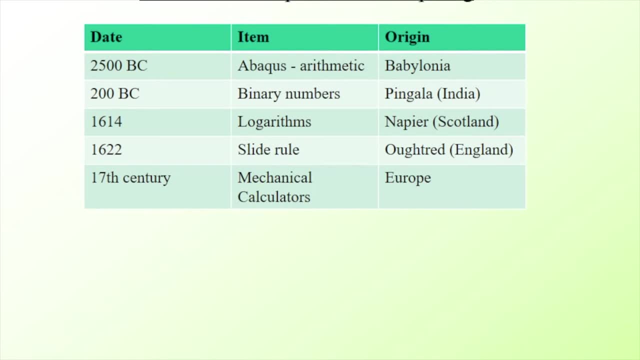 How about historical developments for computing? The first important step was the invention of an abacus for arithmetic in Babylonia 4,500 years ago, no doubt for commerce and collecting taxes. The notion of binary numbers can be traced back to over 2,000 years ago in India. 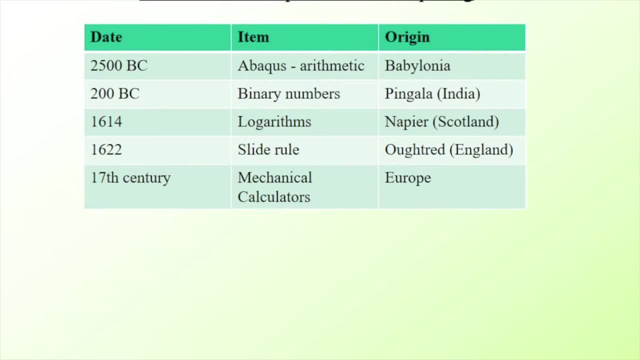 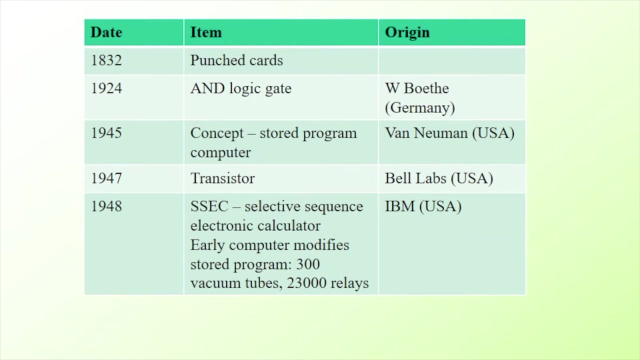 Then in the 17th century, methods and devices of computing were developed. Calculations were developed, such as logarithms by Napier in Scotland, the slide rule and mechanical calculators became widespread in Europe. If calculation is an important aspect of a computer, memory is also a vital component. 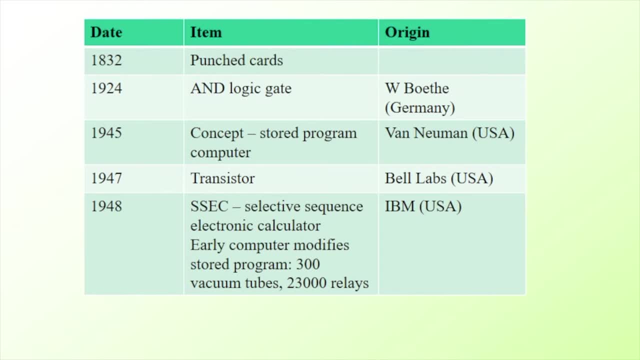 Thus information was stored on punched cards as a concept In the 19th century. the next step was the development by Berta of an AND logic gate, where the output depends on the input of information. So this idea leads to the currently used NAND and NOR gates in logic circuitry. 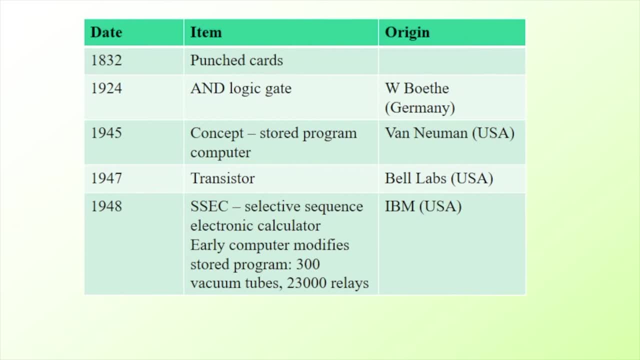 Just after the Second World War, van Neumann introduced the concept of a stored program. Then there was the development of the transistor at Bell Labs. as another crucial step, In 1948, IBM brought out an early computer, which was called a selective sequence electronic calculator, which was based on vacuum tubes and had 23,000 relays. 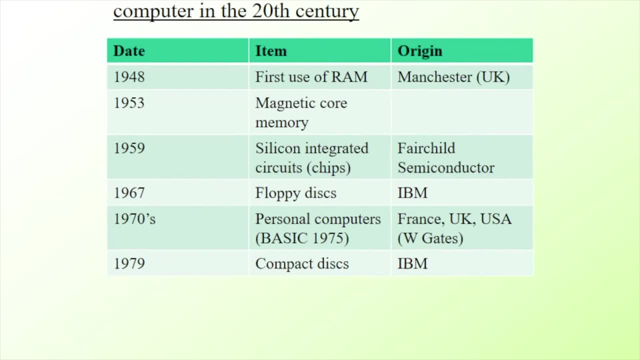 So quite a machine. If early computers were based on vacuum tubes, they were soon to be replaced by silicon integrated circuits with multiple transistors, developed, for example, by far Fairchild. Semiconductor Memory is a crucial aspect of a computer for storing information, and this has seen continuous development through magnetic-based devices such as reels of tape, floppy disks, compact disks and now hard disks. 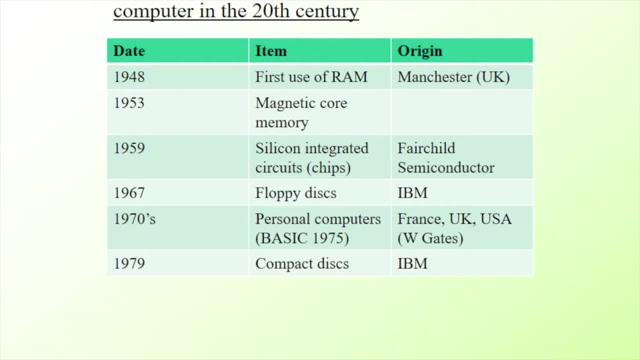 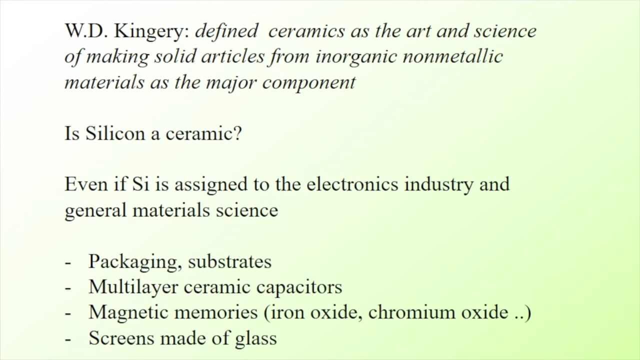 The emergence of the NAND circuitry was the first step. The emergence of the personal computer in the 70s and the 80s on the desk of the scientist and the engineer was a really important step. What about the contribution of ceramics to computers? 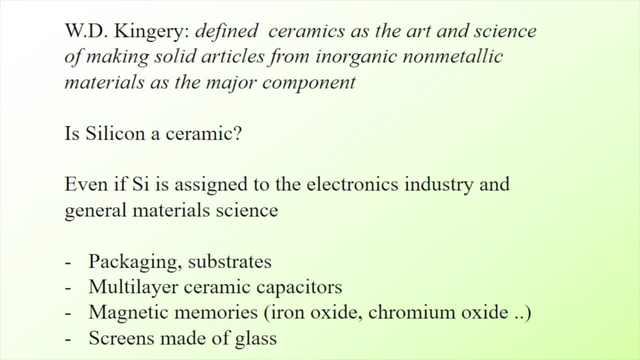 If one takes Kingery's rather wide definition of a ceramic as an inorganic, non-metallic material, one could argue that silicon is a ceramic. In fact, we are now living in a time-traveling age in which, even if we attribute silicon to the electronics industry, we should find various bits of ceramic inside a computer, such as insulating layers, capacitors, memory devices and especially screens made of glass. 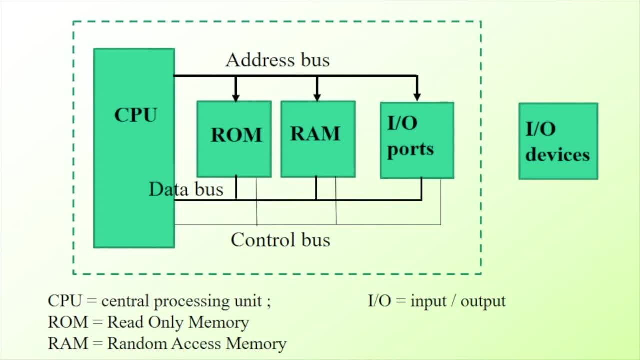 However, our contribution of the ceramics community to computers has been wider than that. This is what I learned as a graduate student at Queens University in Greece. Therefore, I hope what I talked about in this lecture will act as a source of knowledge. vraagtoence Då&a Boeler-K achievementa que fatto a tob let macam que eu tinha escocesas das lemmas vorasmio-ffich otherwise. 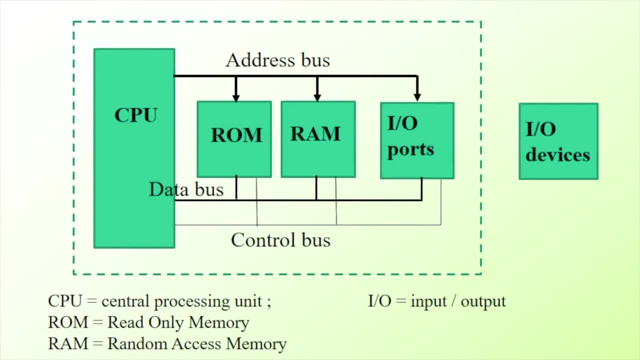 Canada in the early 80s. The microcomputer is composed of a central processing unit plus read-only memory, random access memory and various buses which are connected to the input-output ports which can then talk to input-output devices. Well, the ceramics community contributed the concept of read-only memory over 5,000. 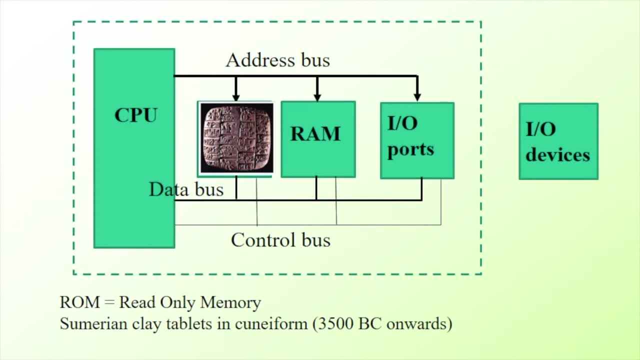 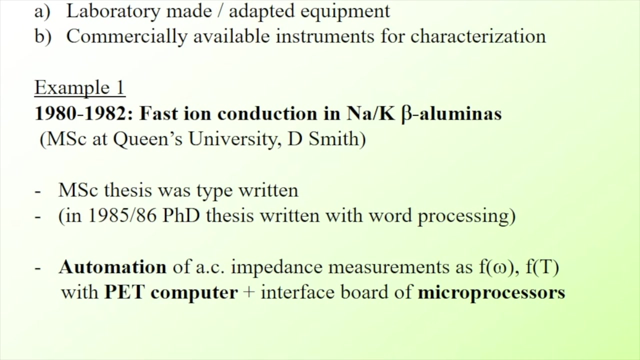 years ago in the form of clay tablets for recording tax information in early Sumerian cities. That's for fun. but we see how important concepts can be found in neighbouring domains of technology. How about the reverse relation on the effect of computing on ceramics? 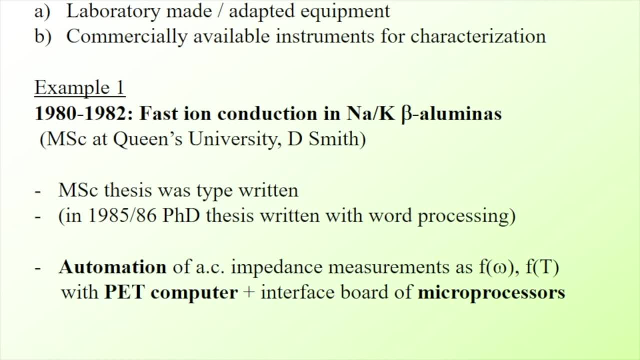 I'm going to start with instrumentation for ceramic science. One can consider the laboratory-made equipment, or we can also consider commercially available instruments. As a first example, I'm going to talk about some work I did 40 years ago on fast iron conduction in beta-alumina. This was my MSc thesis at Queen's University. 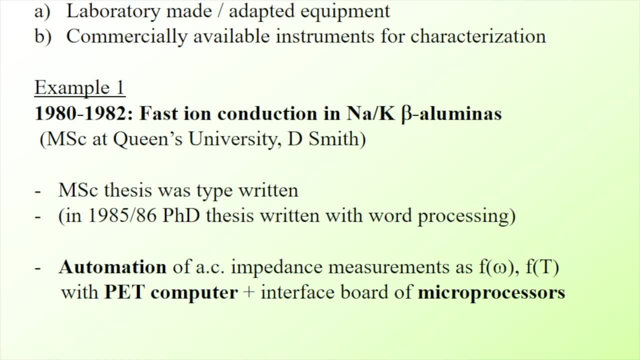 Incidentally, my thesis was typewritten at that time, but when I got round to my PhD, this was written with a word processing package. Anyway, one of my important tasks in this work was the automation of AC impedance measurements for beta-alumina with a PET computer and an. interface board of microprocessors. I'm going to talk a little bit more about that in just a moment, So let's get started. I'm going to start with the first example. I'm going to start with the first example, So let's get started. I'm going to start with the first example. I'm going to start with the first example. 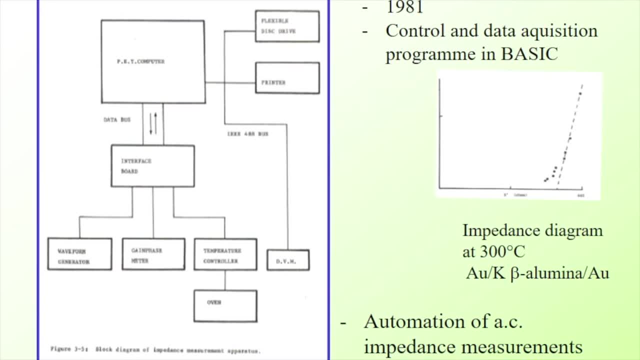 Here is a block diagram of the experimental setup. So we can see that the interface board is linked to the PET computer via a data bus and then it talks to a waveform generator, a gain phase meter to make the measurements and a temperature controller to set the temperature. 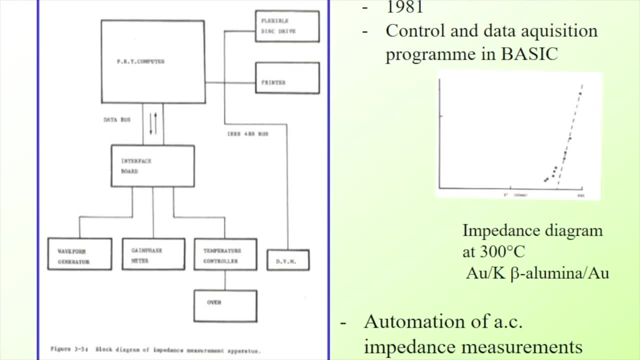 of the oven, in which the temperature of the oven is determined by the temperature of the oven, heits and values are placed. I can see with both hands that three of the different design gauges provide one yield according to each temperature. I see that the temperature of 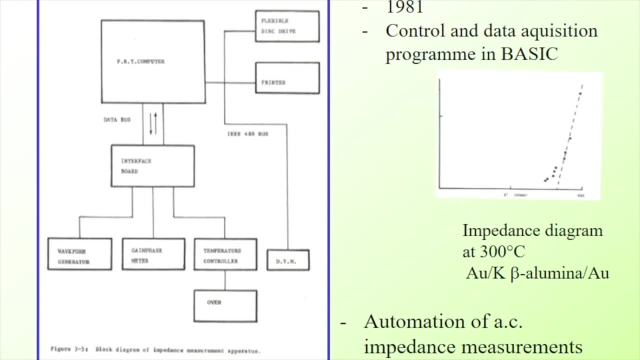 this particular reading algorithm. as well as this one is the equation evento in which the Z current of the pre-코2 latent ringing temperature in fulfill the threshold in which our sample was placed here. So all this was driven with a control data acquisition program. situation program written in BASIC. 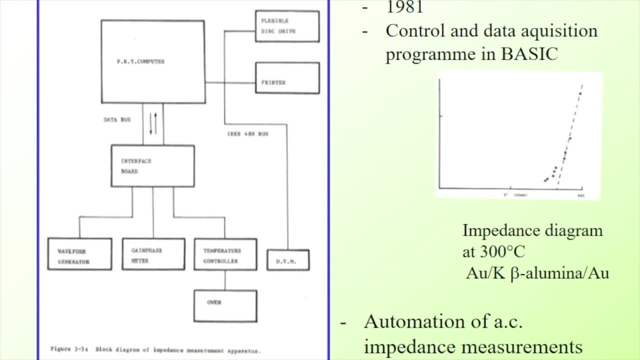 The first, only. basically, This gave us a screen output in real time of the impedance diagram. works quickly, fooling me. very useful to see whether the experiment was working well. Here's the an example of an impedance diagram for blocking electrodes of gold on petacly probe and through lumina. 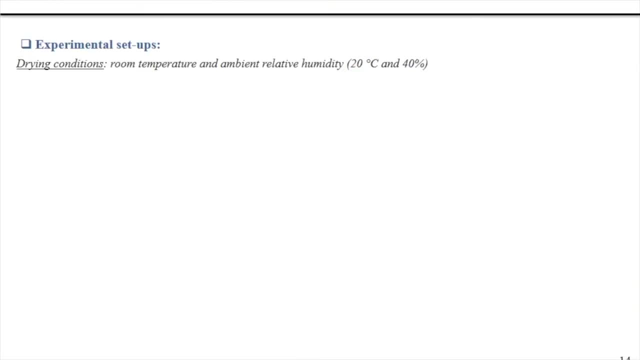 Another more recent example comes from my research group in Limoges, led by Benoit Nathalie, which is working on drying behaviour of green bodies. One method of characterisation that's important in drying is to simultaneously measure mass of the sample and dimension, which is traditionally done with LVDT sensors. 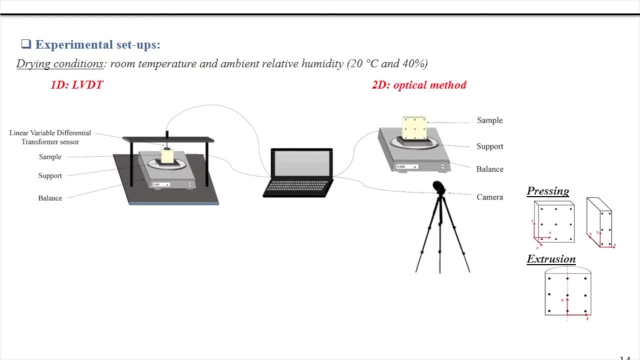 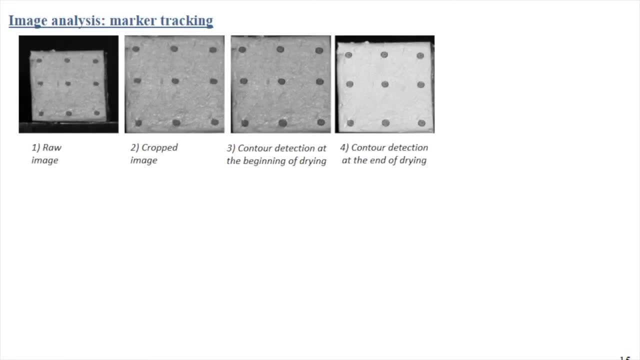 But we've been looking at doing this with optical cameras so that we can get information in two dimensions. Here we can see that the sample has been marked with black dots and these are followed by the camera. Here we can see that the sample has been marked with black dots and these are followed by the camera. 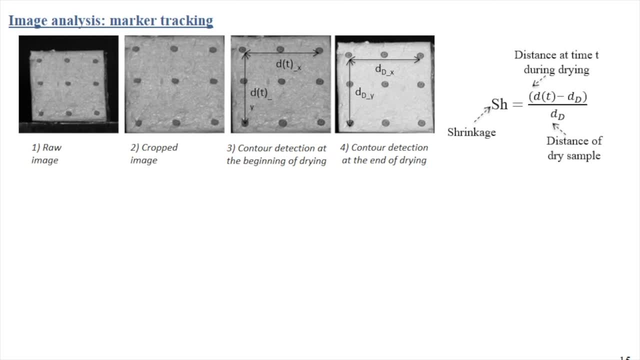 It's actually happening for 2 parts in the experiment. We have a computer programme which is written in Python, which evaluates the distance between these dots as a function of time. It crops the image first and then it works out the contours of the dots and then the 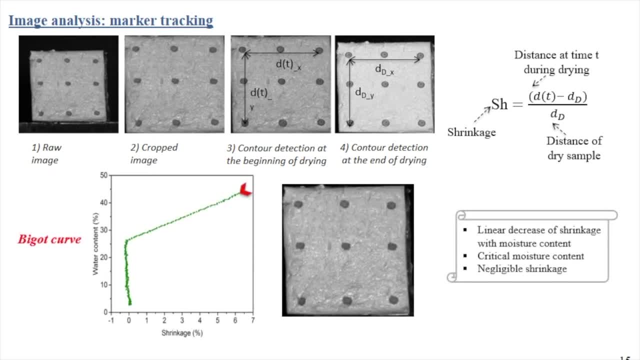 distance between these dots. As an example, here we can see that there are two phases in drying, where there is shrinkage, and then when the green body has become rigid. we then have a second phase, where water is still being taken out of the sample, but the sample is no longer evolving in dimension. 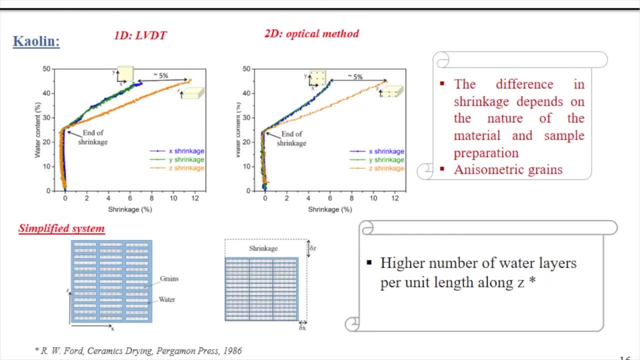 Here in this slide the two methods are compared for kaolin ceramic, which has anisotropic shrinkage, You can see that this is well registered with the 2D optical method, but with one experiment. This anisotropic shrinkage can be explained by the preferential orientation of kaolin platelets, which gives different numbers. 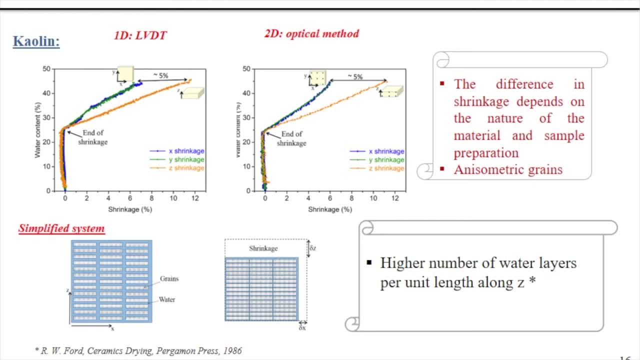 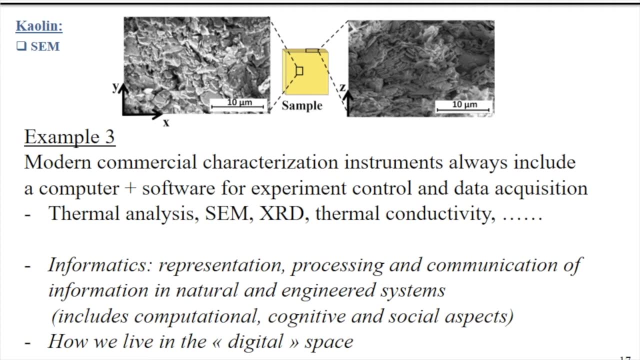 of water layers according to the direction. In this final micrograph we can see that the kaolin platelets are indeed preferentially oriented. A third example that I would like to consider is if we look inside the laboratory, we will find lots of different characterization instruments, like 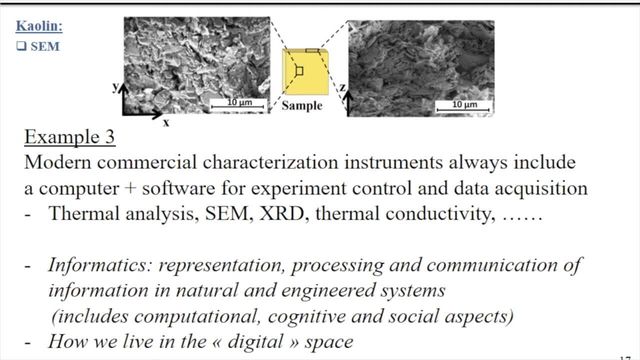 thermal analysis, electron microscopes, x-ray diffraction equipment, thermal conductivity equipment, All of them will have a program, a computer program, a computer and a computer program to drive them and also to help the data acquisition and analysis. So here I've put up a definition of 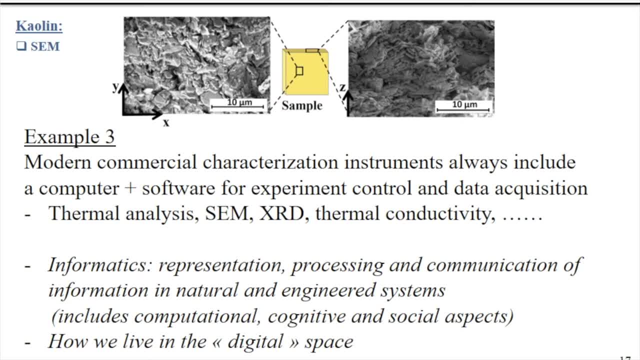 informatics, which is representation, processing and communication of information in natural and engineered systems, or, if you like, how we live in the digital space. but what we can say is that computers have become an indispensable tool for instrumentation. I now want to look at modeling of synthetic ceramics. 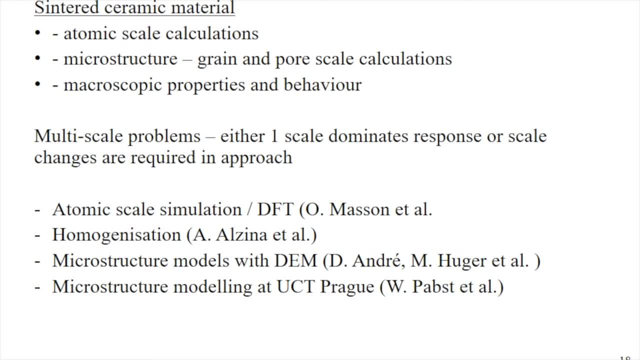 definitely computational material science. Models are made at different scales: the atomic scale, the grain and pore scale or even the macroscopic scale for general behavior. Either one scale is going to dominate, or else we have to handle in some way scale changes. 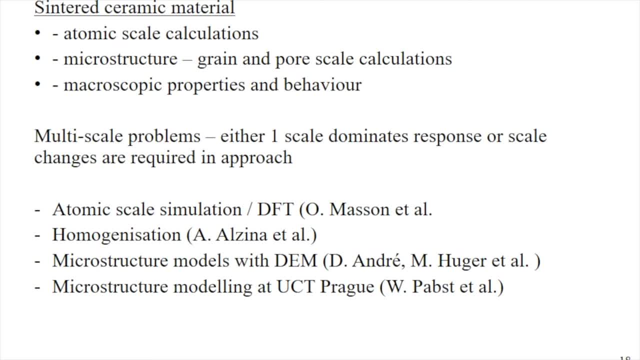 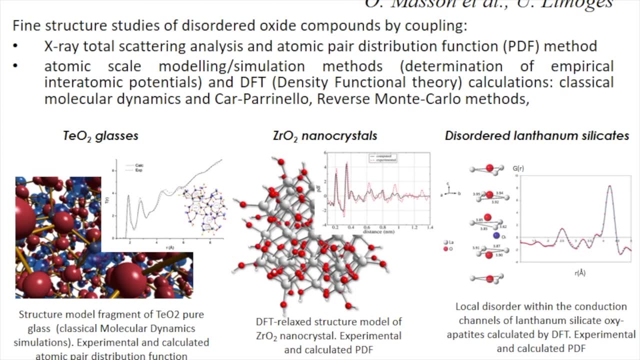 So here are a few examples which we're going to explore. Olivier Masson's group in Limoges are specialists in making atomic scale models. They use in particular x-ray total scattering analysis to get the atomic pair distribution function and then they're able to do density functional theory calculations to make a model of the structure. 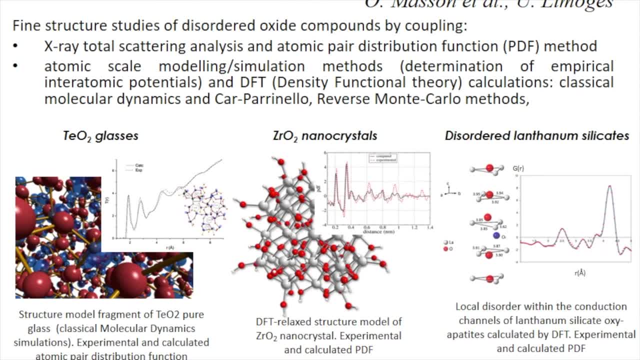 So they've been working on tellurium oxide glasses, zirconia nanocrystals and disordered lanthanum silicates. We're going to focus in briefly on lanthanum silicate. The interest of their approach is to make a model of the structure of the atom. 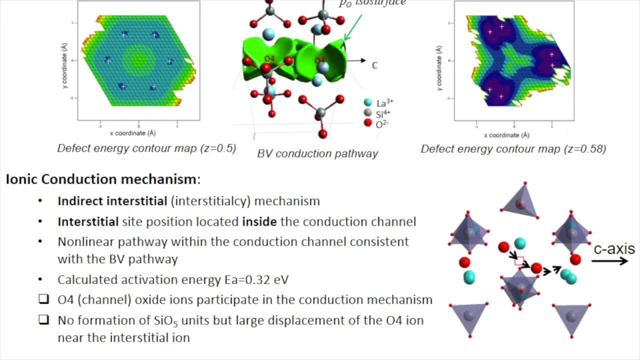 I'm going to show you a few examples. The first example is for ionic conduction and to predict the conduction pathways and, in particular, what activation energy the ionic conduction would have. So this is oxygen ions and with potential for fuel cells. In my second example I want to illustrate 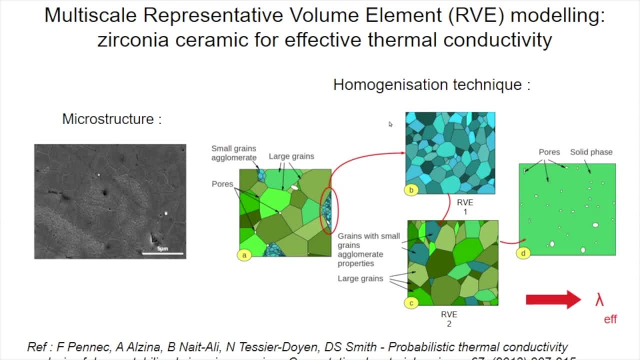 modeling done at the grain scale, at different scales, So the homogenization technique. This is the case of zirconia ceramic with two different grain sizes and pores. We can see this in the micrograph. So there's a representation of this in the first schematic of the. 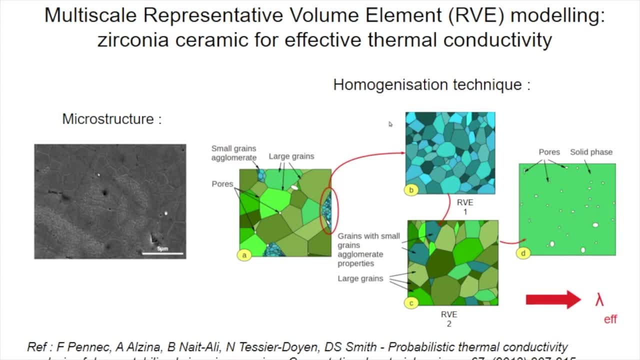 microstructure. Then, in terms of a representative volume element, we'd have a first stage where we calculate the solid phase thermal conductivity, taking an average value over the small grain and large grain regions, And then this is a ceramic model. This is an example of a 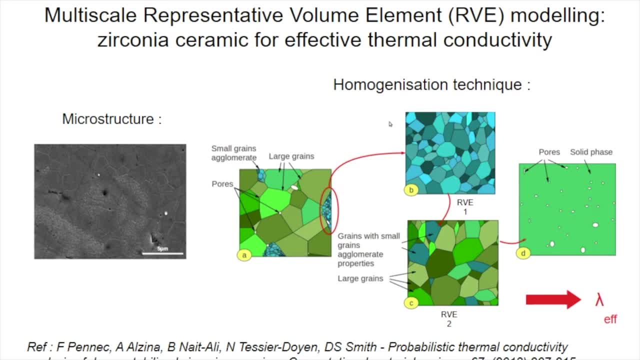 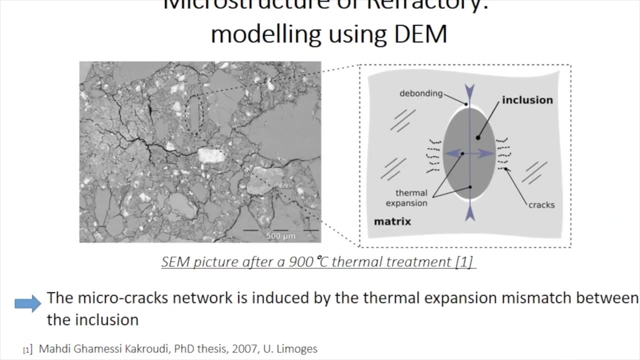 combined in a second step, where we take the solid phase thermal conductivity and combine it with that of the pores, And so this will give us an overall thermal conductivity. In another example concerned with mechanical properties, Marc Houger's group has been looking at the complex microstructures of refractories. 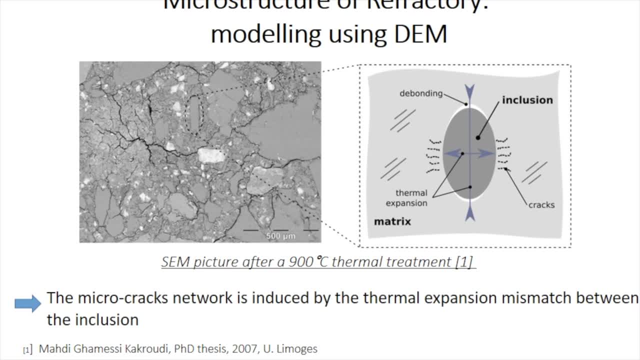 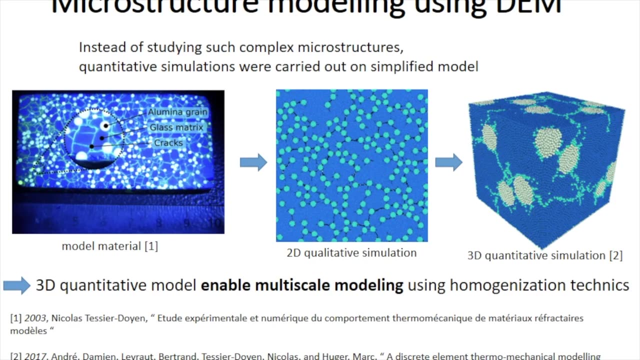 In this particular case we have a mixture of solid phases And, because of the difference in thermal expansion coefficients, cracking and deep bonding can occur. The approach has been to simplify the system and to use a model material, So in this case it's a mixture of alumina inclusions in a glass matrix. 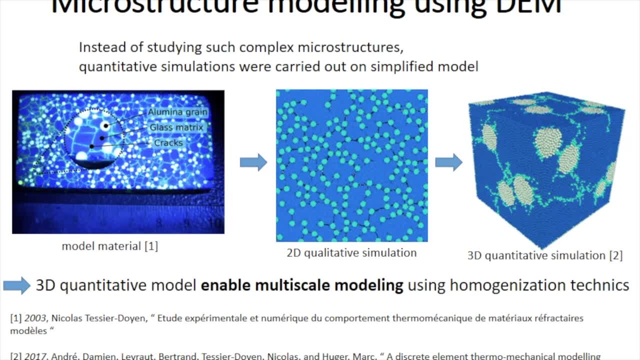 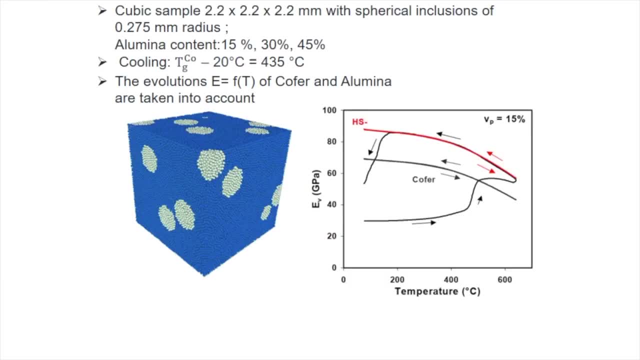 where the glass matrix can be chosen with different thermal expansion coefficients. In particular, Damien Andre has been carrying out discrete element calculations on the system. So in the first case he's got the thermal expansion coefficient for the matrix which is stronger than that of the inclusions. 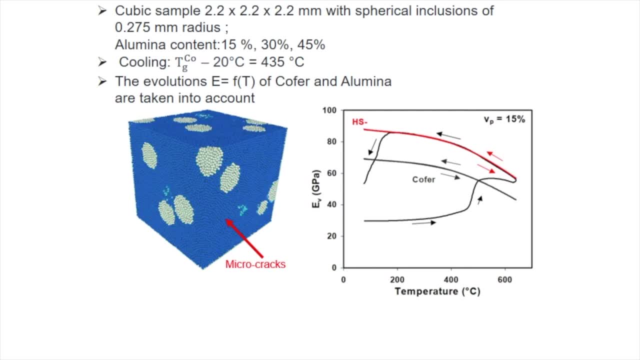 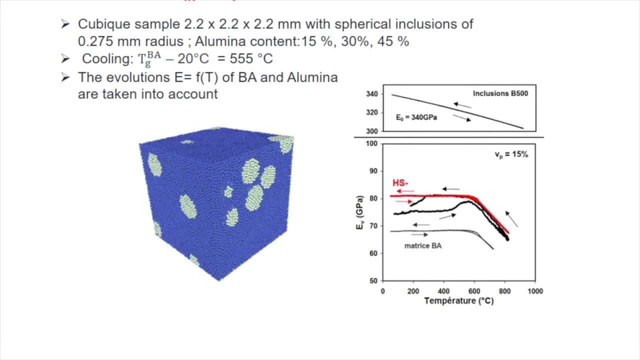 And if we look at the simulation, we can see that microcracking occurs. In the reverse case, where the matrix thermal expansion coefficient is less than that of the inclusions, the effect is different, And what we now get is deep bonding. 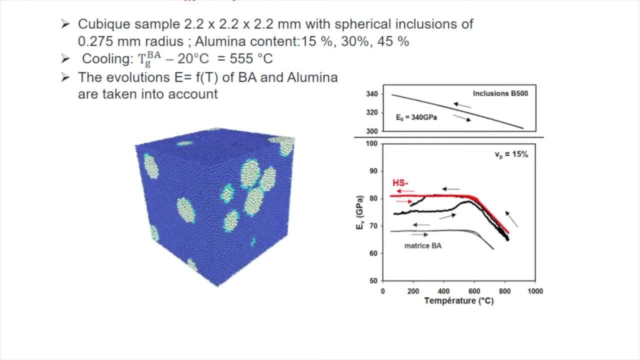 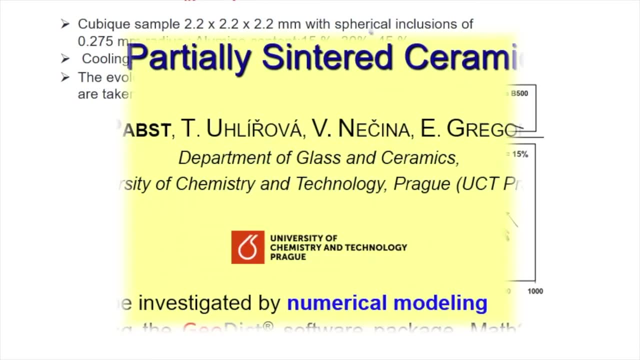 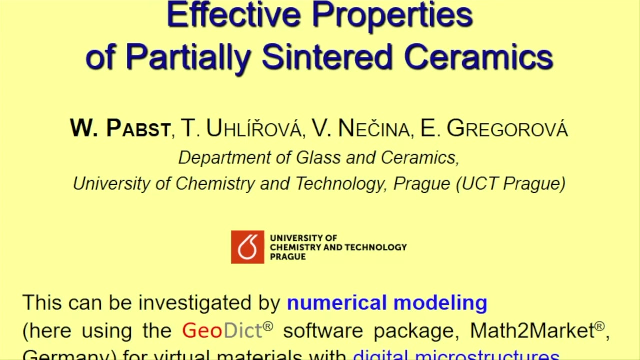 so space between the alumina inclusion and the matrix. My final example in this section is from the work of Woody Papp's group in Prague on thermal and mechanical properties. After a lot of work on porous ceramics, they have been looking at partially sintered ceramics. 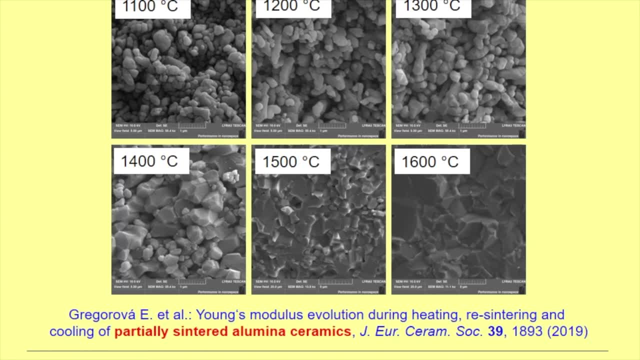 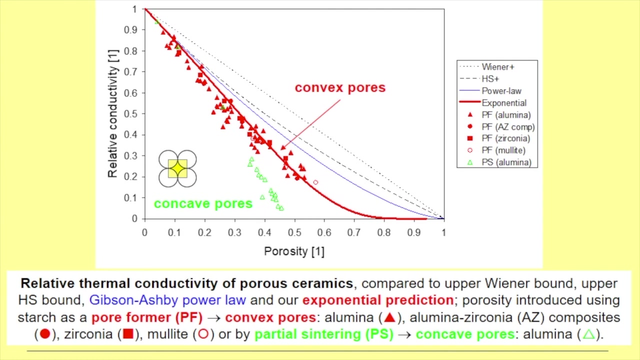 In essence, the microstructures of these partially sintered ceramics reveal rounded or convex grains and concave pores. Well-known analytical models for thermal conductivity of the porous ceramic are based on convex pores, such as the Haschen-Strichmann upper bound. 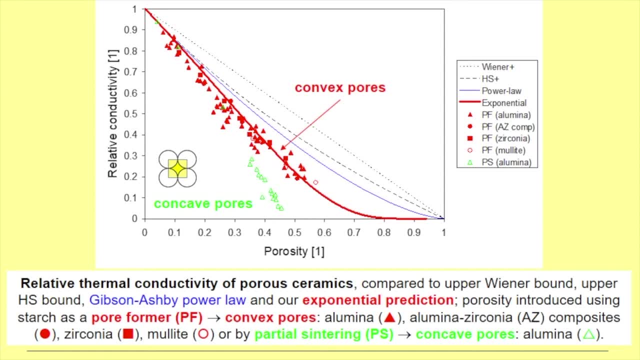 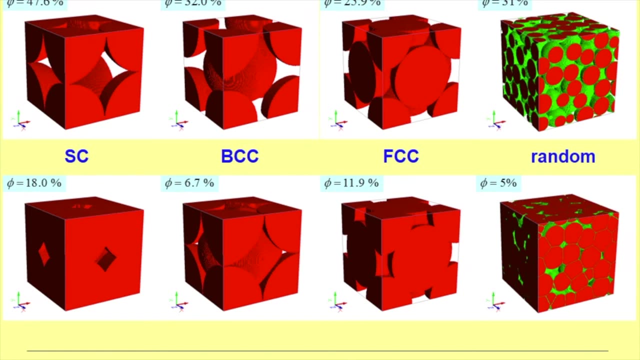 or equivalent to the Max-Leukin relation. But experimental data on the partially sintered ceramics yield values in green beneath these predictions. So Woody's group have been using the GeoDict software package to explore the effect of concave pores on the thermal conductivity. 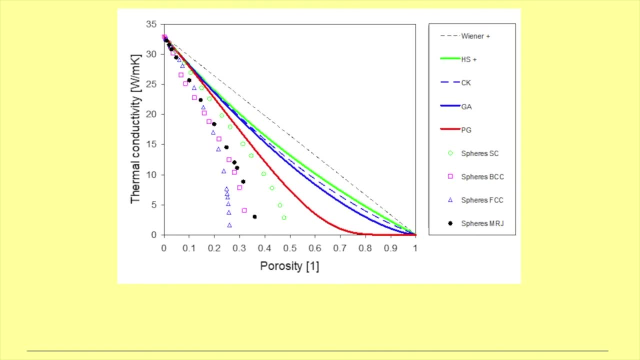 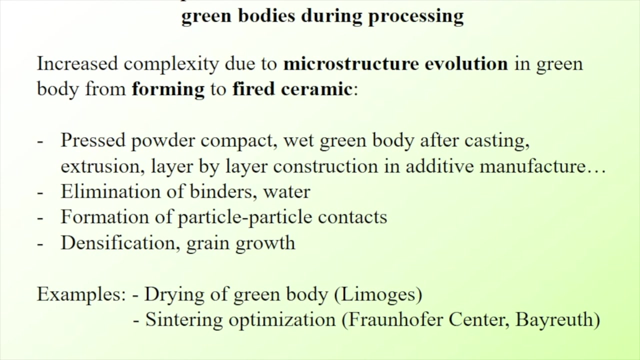 Their predictions are distinctly beneath those of the standard analytical relations and consistent with the experimental data. So the previous set of examples show how refined computer models of ceramics with staple structures can be. The next challenge is to look at green body behaviour during processing. The important point is that, after forming, the microstructure evolves as we go through. 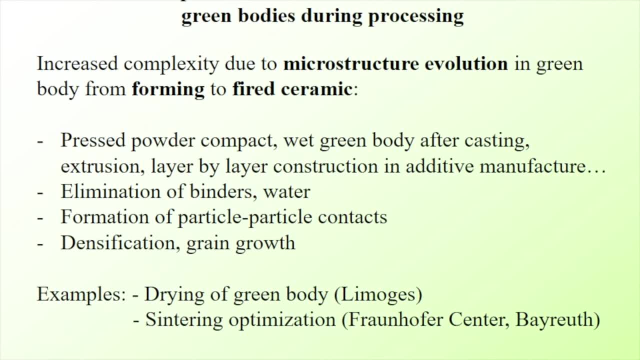 elimination of binders or water, formation of particle-particle contacts, densification and grain growth. We're going to look at two different examples, one on drying and one on sintering. So we're going to look at two different examples, one on drying and one on sintering. 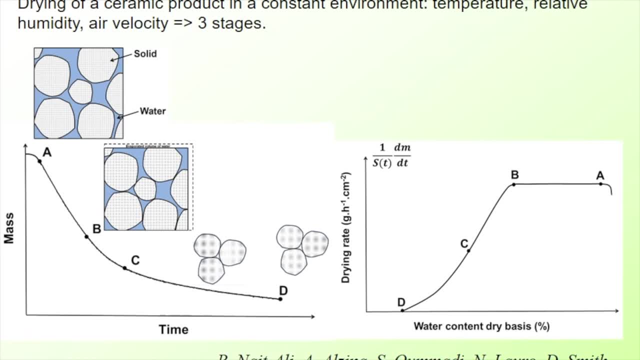 The drying of a wet green body involves at least two stages. The first stage, known as the constant rate period, involves significant shrinkage as water is evaporated from the surface of the sample. Then the drying rate slows down as water is extracted from deeper and deeper in the body. 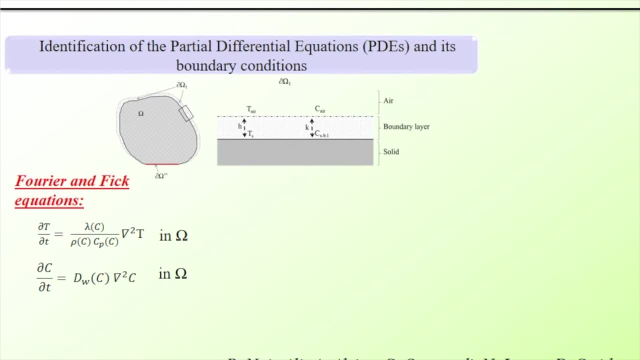 In terms of modelling, one has to solve at least two partial differential equations: One, a heat transfer equation which is coupled to mass transfer. But there is a further complication, and that is that the physical parameters which are found in these equations, like thermal conductivity, diffusivity of the water, 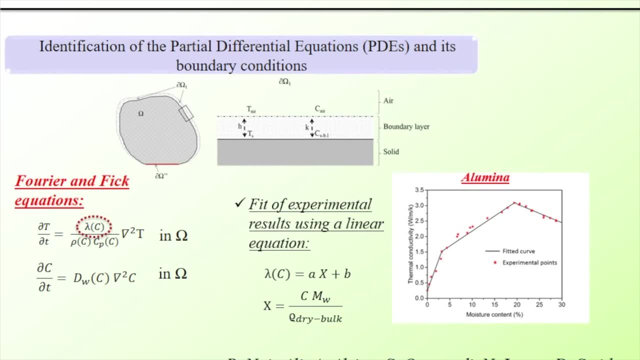 and the temperature of the surface of the sample, The thermal conductivity of the sample and the diffusivity of the water. The thermal conductivity of the sample and the diffusivity of the sample, Mass transferlya and the thermonuclear activity vary with the water amount. 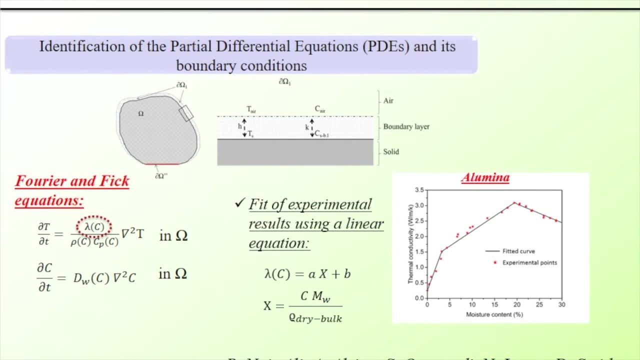 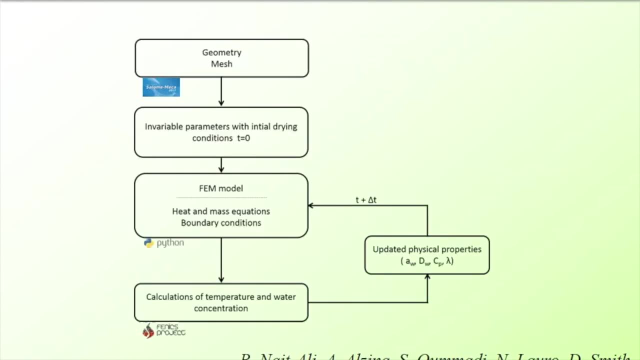 Mass transferlya and the thermonuclear activity vary with the water amount. We can see for Illumina the variation of thermal conductivity with moisture content quite dramatic. So the model has to update these parameters in the calculations as we go through the loss of water. 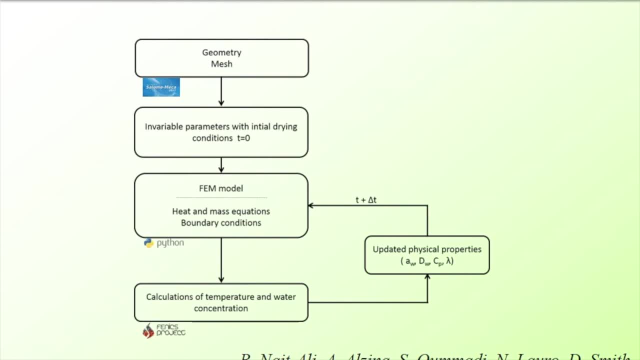 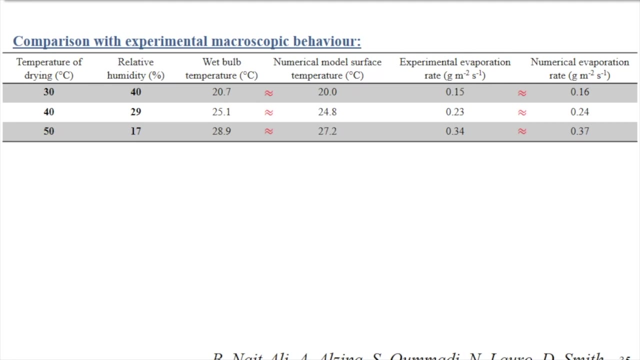 And here you can see that, on the basis of a finite element model, a much more precise study is carried out in our organigram how these physical properties are updated. By doing this, the computer model based on finite elements can predict the drying rate. 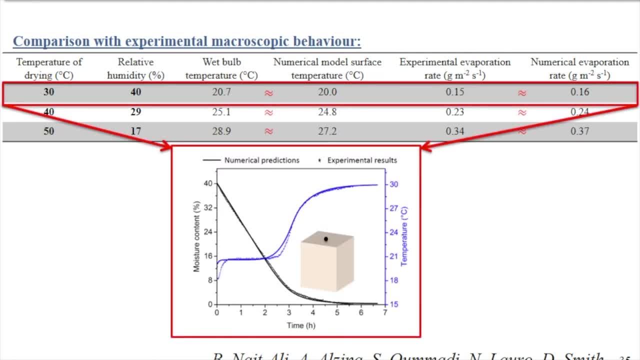 and also the surface temperature as a function of time. These predictions have been compared to experiment and are quite good. However, this is a work in progress, because ideally one wants to get information on internal stress in the body as well, So this would be the next challenge. 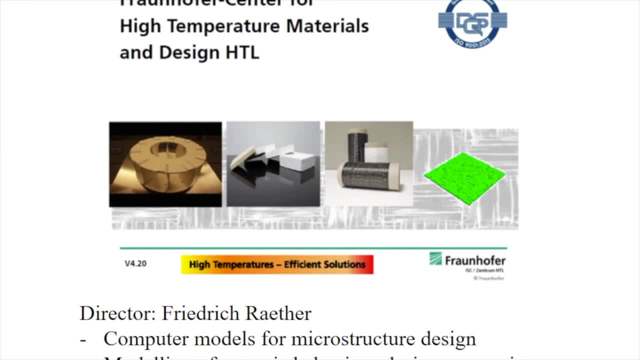 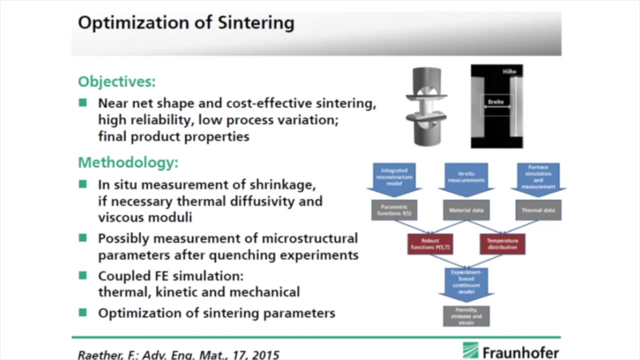 Another example of obvious interest is sintering behavior. Friedrich Rether's group in the Fraunhofer at Bayreuth have been working on computer models for some time. Their mythology has been to combine experiment with finite element calculations and the use of finite element calculations to calculate the temperature of the body. 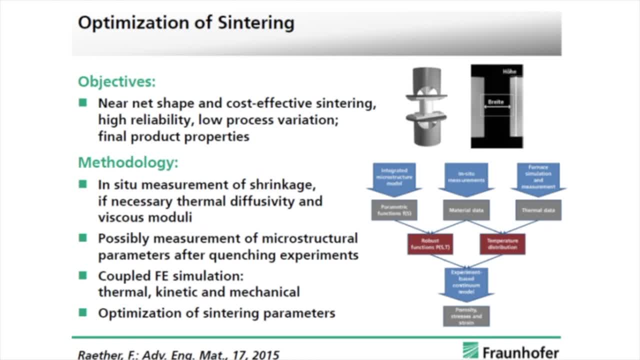 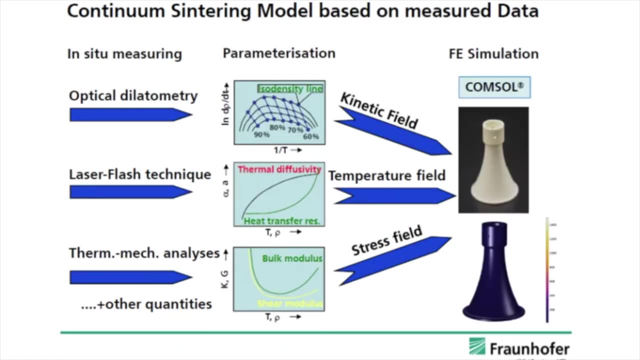 In particular, they have been able to develop in-situ measurements by optical dilatometry and thermal diffusivity. By calculating the temperature field, they can then calculate the local densification of the ceramic in a continuum sintering model, and this has application to complex shapes and even stress. 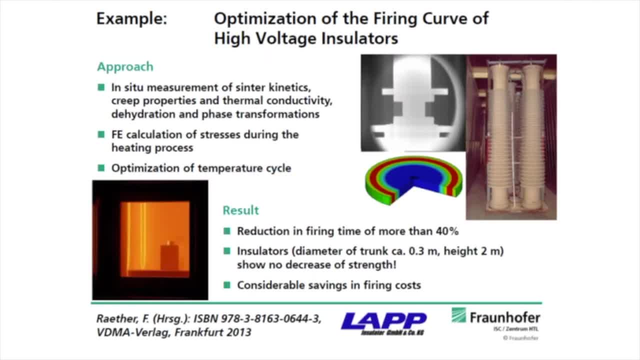 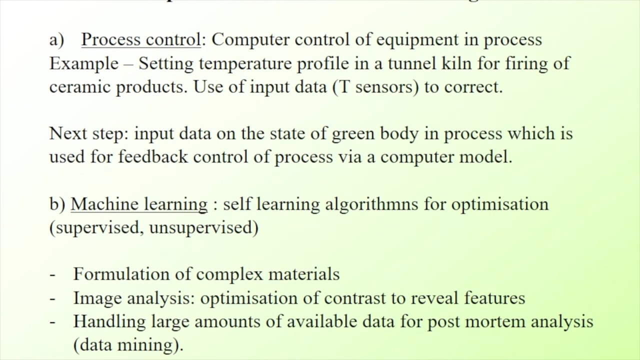 This is the large scaleís calculation of sintering behavior. The study has already performed some research and this has been used to optimize firing of high voltage insulators. The study has led to a reduced firing time and hence reduced costs. Just to finish up, I want to mention two domains with prospects for the future.